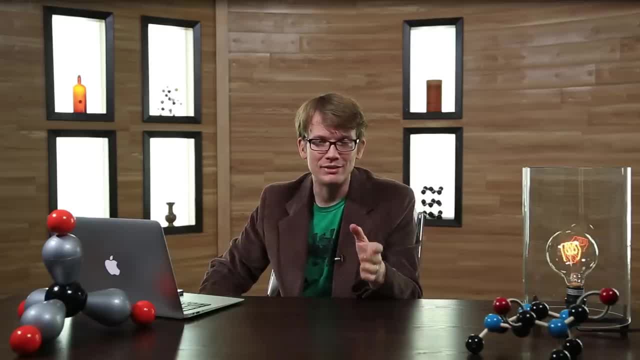 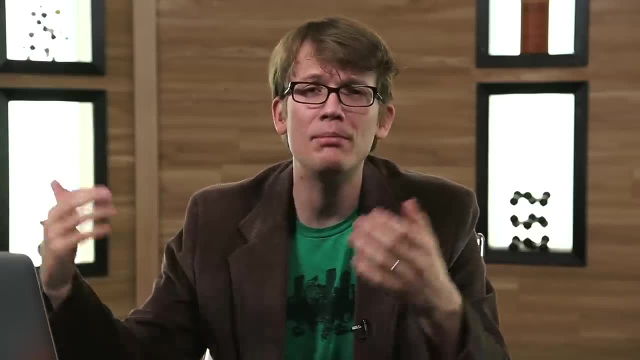 Hello, I'm Hank Green and I want to teach you chemistry, But please do not run away screaming. If you give me five minutes to try to convince you that chemistry is not torture but instead the amazing and beautiful science of stuff, and if you give it a chance, it will not only. 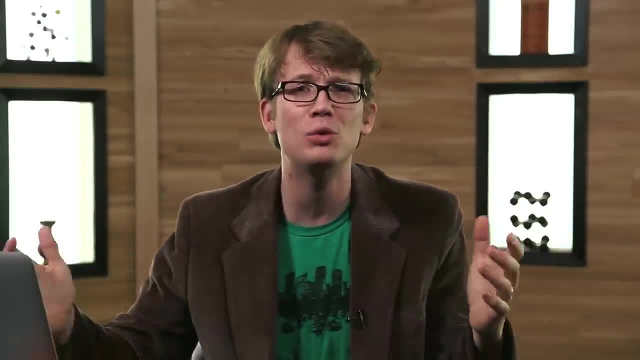 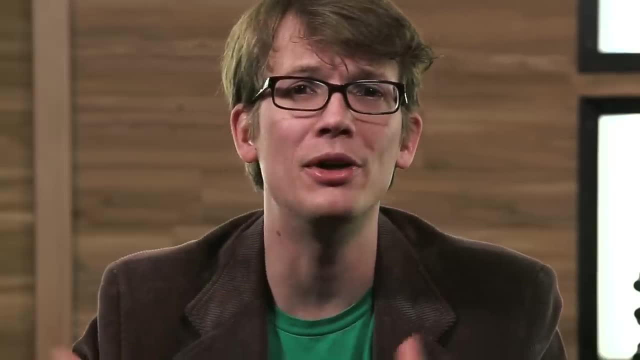 blow your mind, but also give you a deeper understanding of your world. This is just my opinion here, but I think that understanding the world leads to a greater ability to enjoy the world, and there's nothing that helps you understand the world better than chemistry. 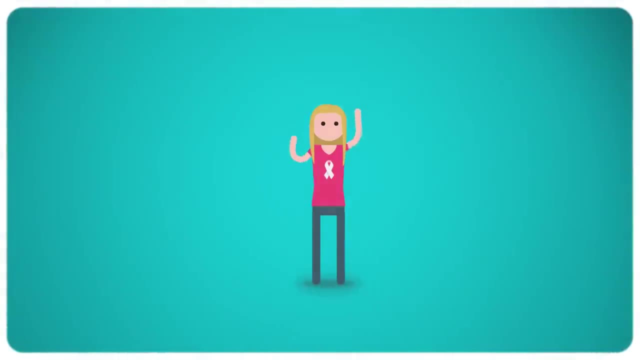 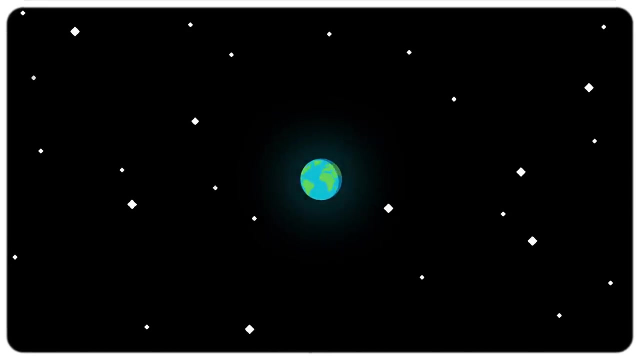 Chemistry holds the secrets to how life first formed, how cancers are cured, how iPhones have bigger hard drives than five-year-old laptops and how life on this planet might just be able to continue thriving- even ours, if we play our cards right. 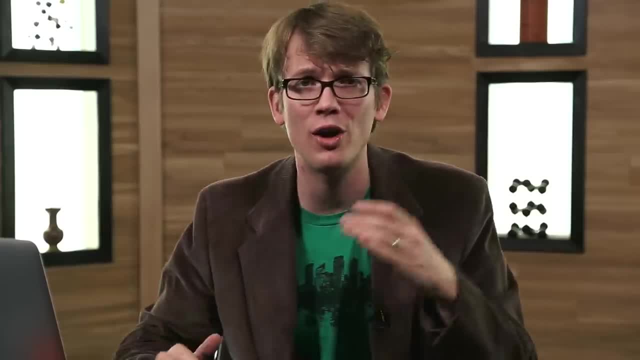 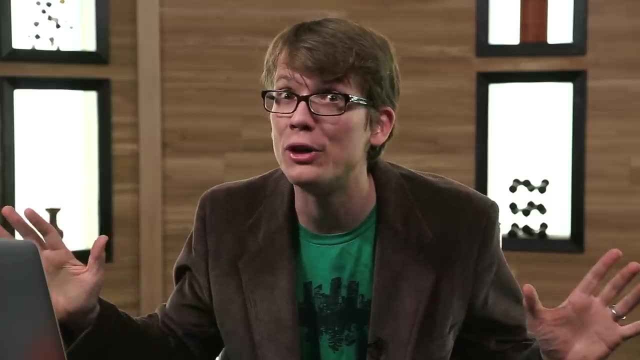 Chemistry is the science of how three tiny particles, the proton, the neutron and the electron, came together in trillions of combinations to form. get this everything Now. chemistry is a peculiar science. It's sometimes talked about as a bridge between the ultra-abstract world of particle. 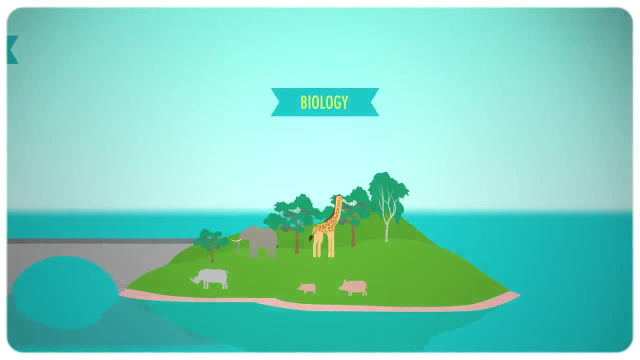 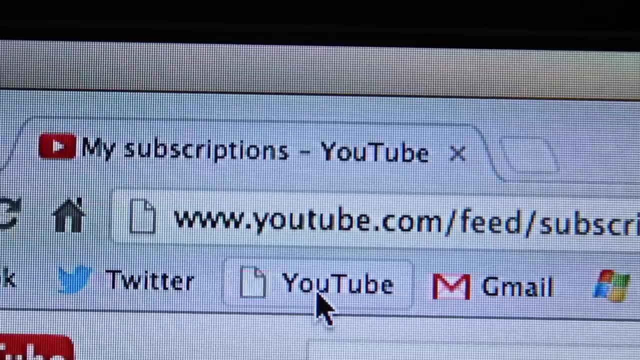 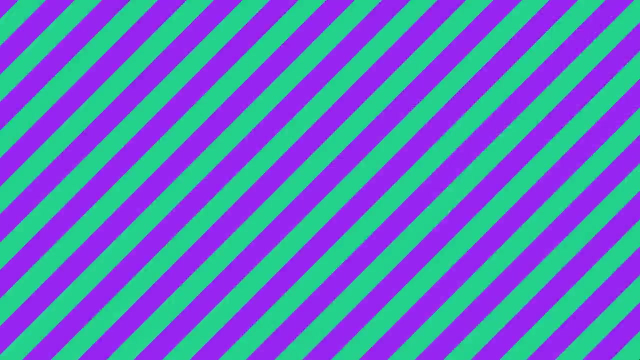 physics and the more visible sciences like biology. But calling chemistry a bridge is like calling Eurasia an island. Chemistry has it all: Mad scientists, world-changing revelations, the practical, the impractical, medicine, bombs, food, beauty, destruction, life and death. 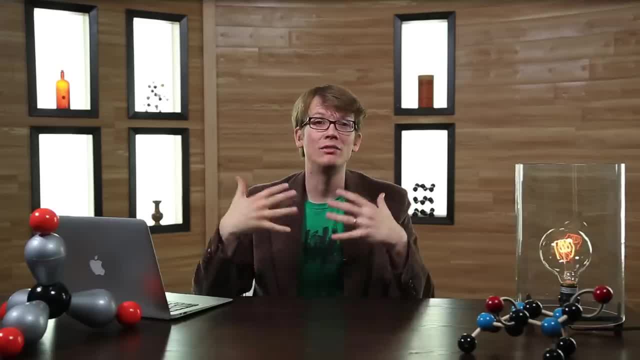 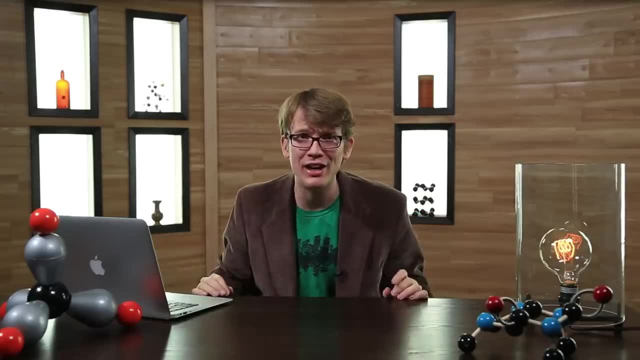 Answers to questions you never knew you had. I love chemistry and I hope I can give you a glimpse into why. So today let's talk about it. Let's start out with maybe the biggest idea of all time and move on from there. 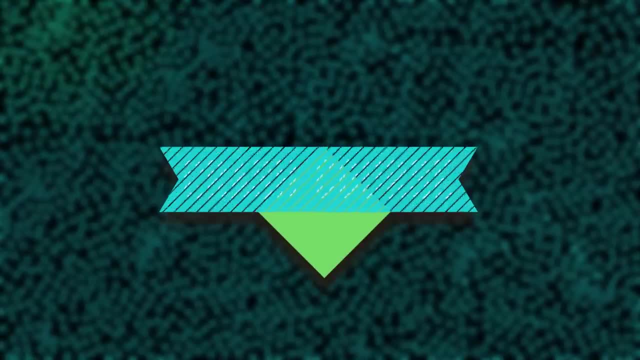 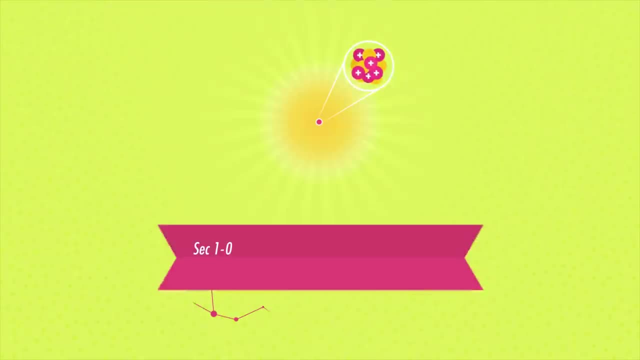 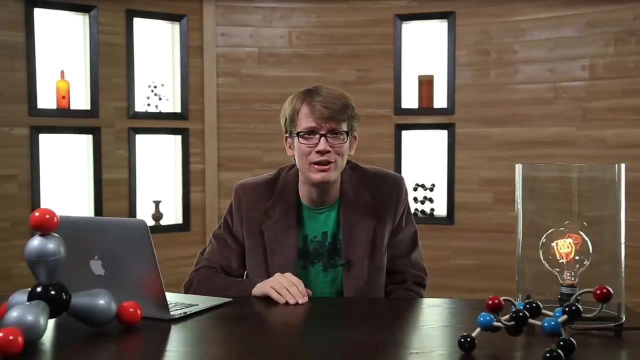 Stuff is made from atoms. I know you aren't shocked, You aren't awed, You might not even be paying attention anymore, But when atomic theory was first proposed it sounded pretty crazy. And, yes, we call it atomic theory. 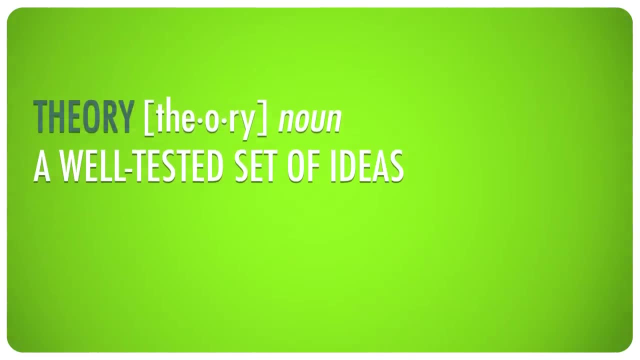 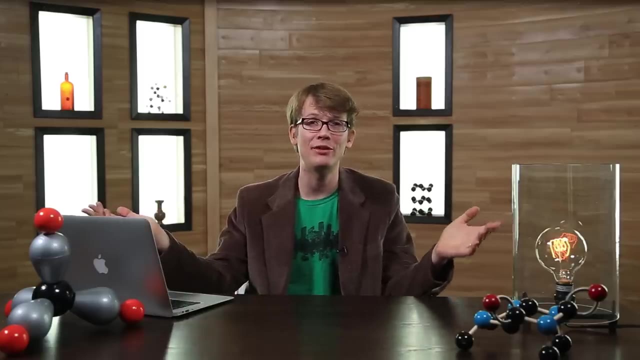 It's the scientific definition of theory, which is a well-tested set of ideas that explains many disparate observations, not the colloquial definition of theory, which is a guess, Though luckily there's no one running around anymore saying atoms are just a theory. 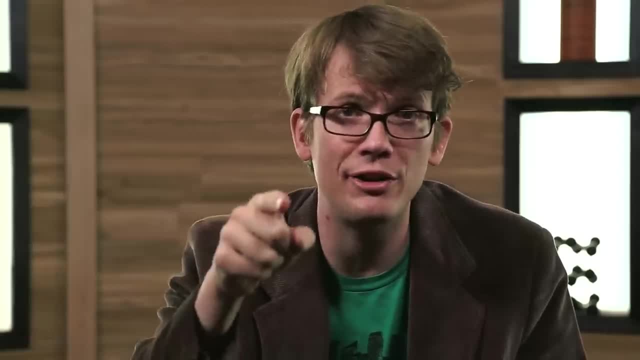 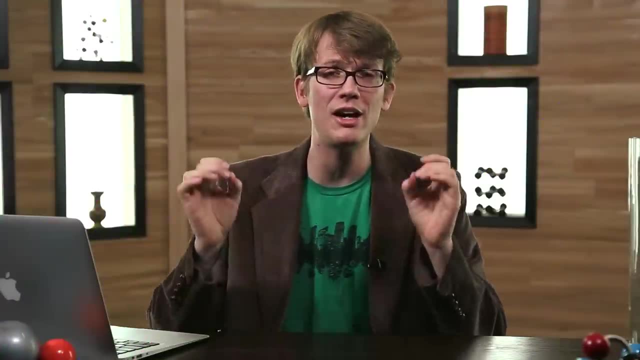 But it wasn't that long ago that people were running around saying that, and you want to know who settled it for good, Einstein. Atoms had been postulated for a long time, by the 20th century, but it wasn't until Einstein mathematically proved the existence of atoms and molecules in 1905 that the matter 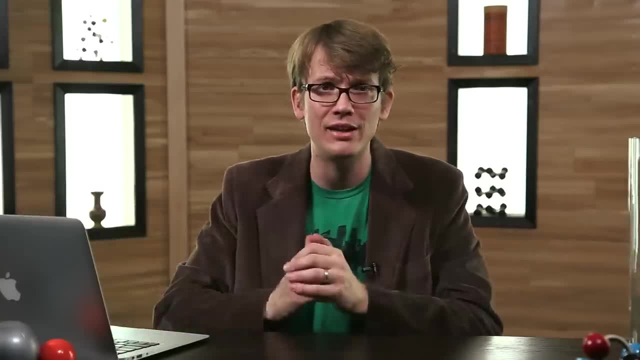 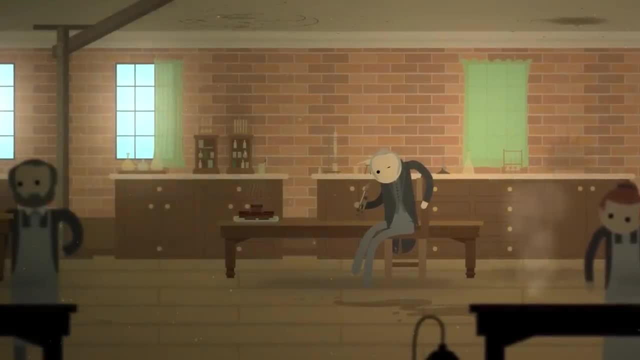 was truly settled And you thought Einstein was all about relativity and E equals mc squared. He also proved atoms exist. Here's how it happened: In 1827, a botanist named Robert Brown was looking at pollen grains in water through. 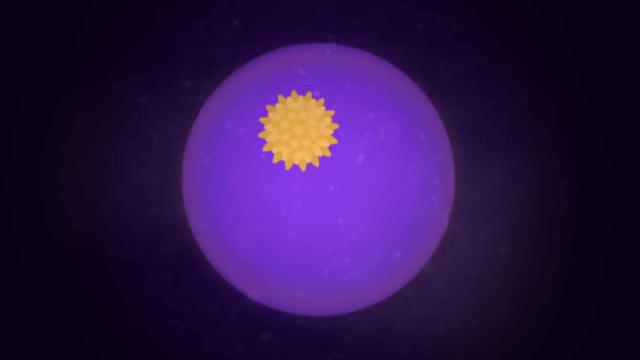 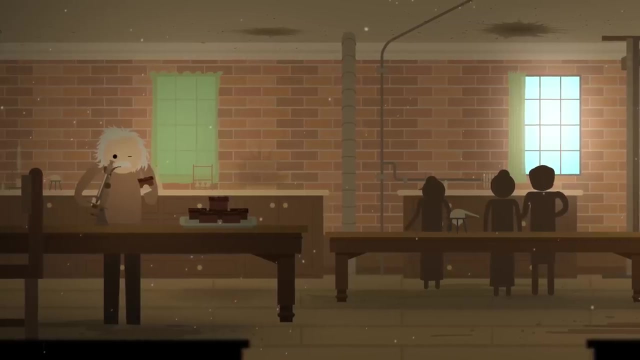 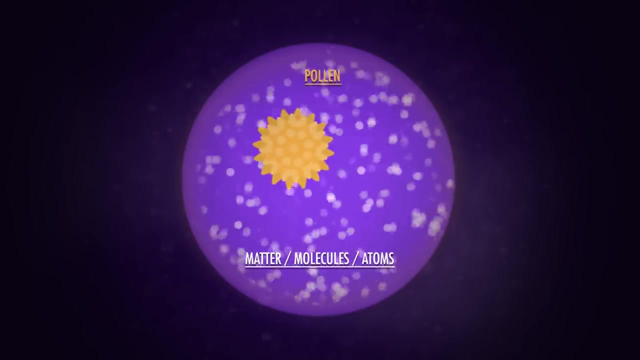 a microscope and he noticed that they jiggled randomly even when there was no movement. to cause the jiggling It was a mystery for a long time, until 1905, when Einstein theorized that this phenomenon was caused by as-yet-unproven atomic particles actually smacking into the grains of pollen. 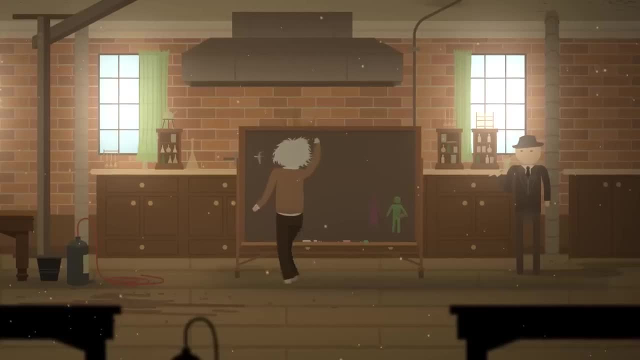 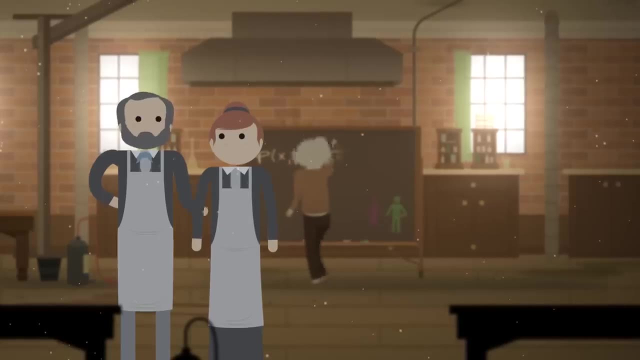 He wrote up some fancy math showing that his theory predicted this motion almost perfectly, and everyone had to concede that, yes, tiny, discrete bits of matter were indeed smacking into the pollen, and thus molecules and, by extension, atoms must exist. 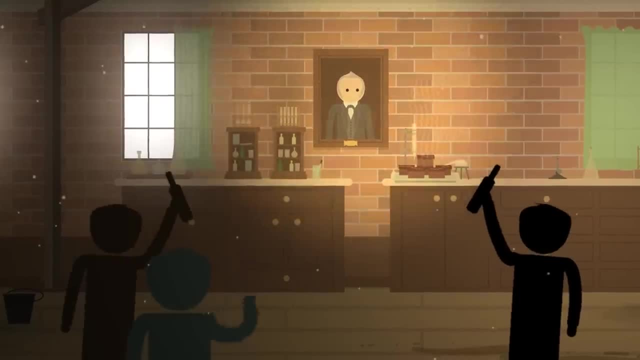 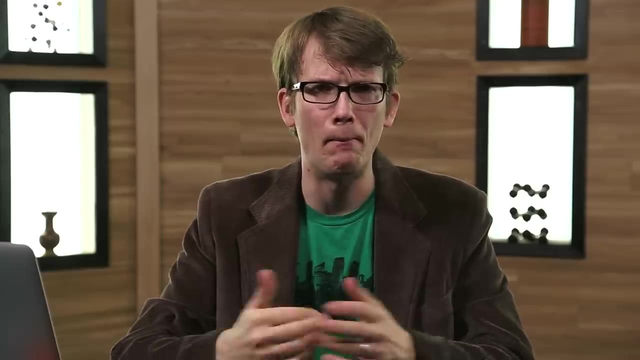 Today we remember this botanist and his discovery by calling the motion he observed Brownian motion. It's kind of crazy that every physical thing you've ever interacted with is made up of little ball thingies. It started with people wondering what's going on. 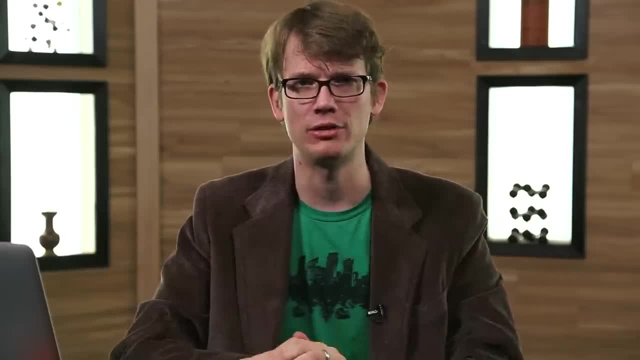 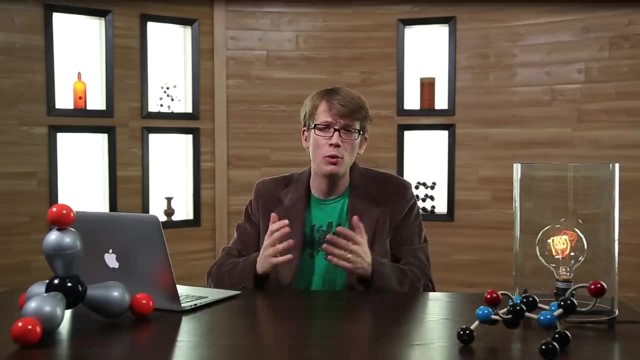 What would happen if you just kept slicing something in half forever? Eventually- and of course it turns out that there's no knife sharp enough to do this- you end up with one pure, unbreakable bit of that substance. The word atom, indeed, is from the Greek for indivisible, though of course, as we learned, 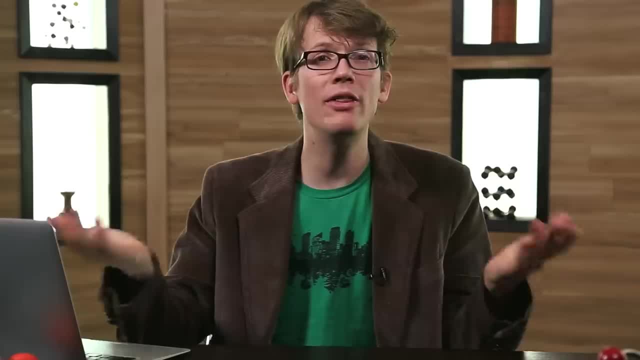 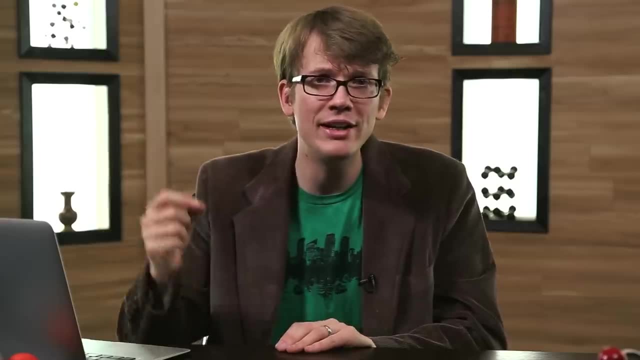 in World War II. atoms can be broken as well, So all the stuff that we think of as stuff is made of atoms: tiny, discrete particles that have specific properties depending on the arrangement of three simple subatomic particles. There's the proton. 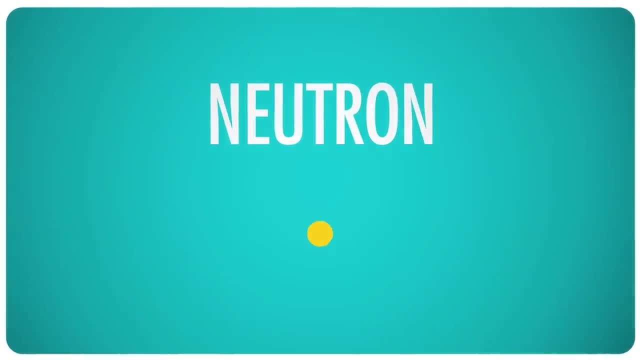 The proton is a particle that can be any size and positively charge. the neutron, about the same size as the proton but neutral. And the electron, which has the same amount of charge as the proton, just opposite, and very nearly has no mass at all, about 1800 times less massive than the proton or neutron. 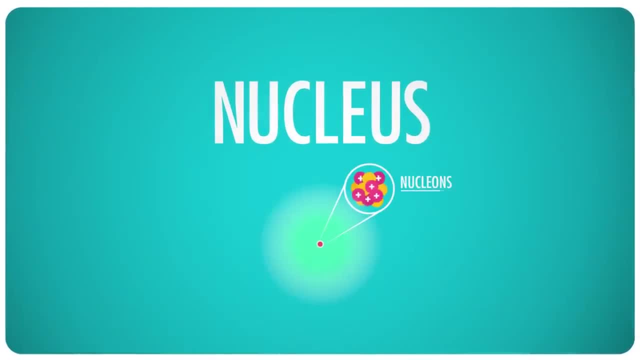 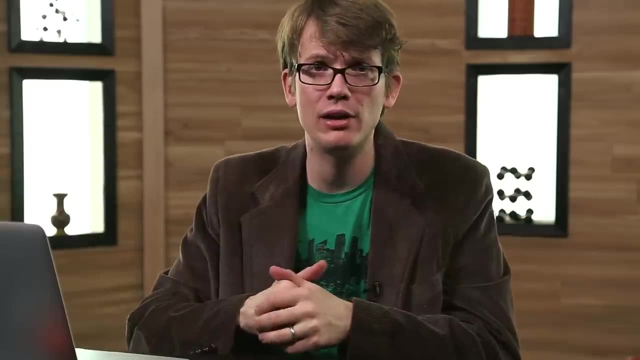 Protons and neutrons hang out in the nucleus and thus are the nuclear components, or nucleons. Electrons hang out around the nucleus and are the parts of the atom that do all the interesting chemical stuff. But before we get to the chemistry of the electrons we first have got to understand. 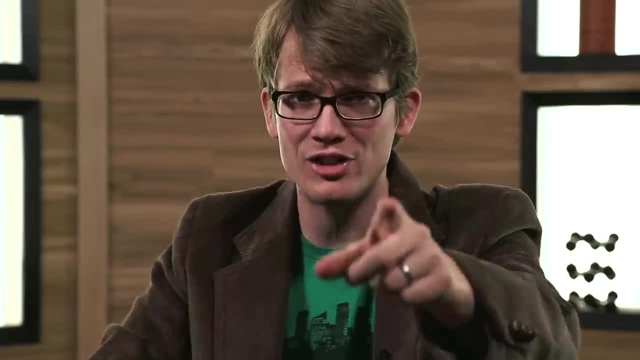 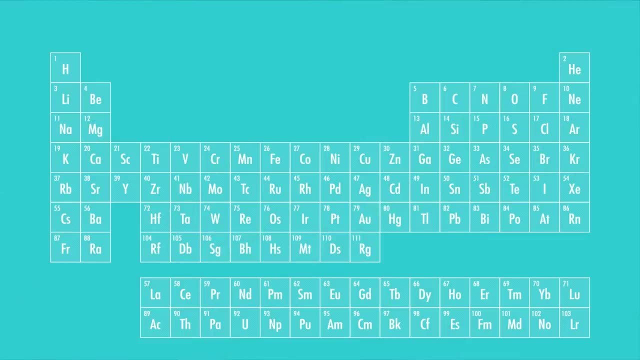 the properties of the nucleus. Okay, this is pretty important, so pay attention here. The number of protons in an atom determines what element it is: 79 protons always gold. 59 protons always praseodymium. 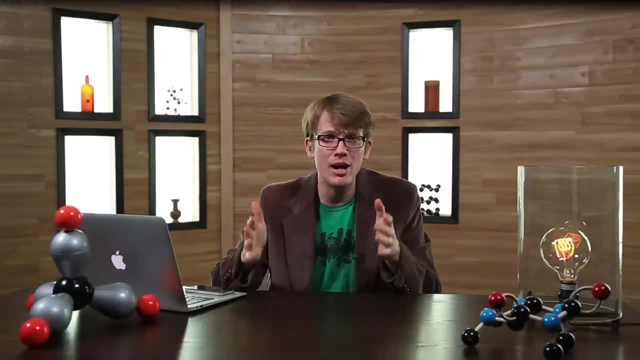 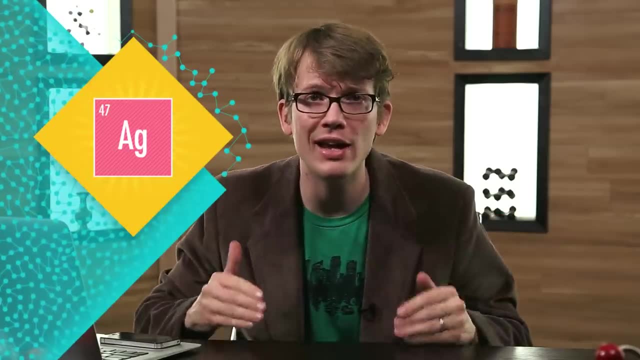 The number of protons in an element is its atomic number. It sits right on top of the box in the periodic table because that is the element's defining trait. So an atom of silver with 47 protons in its nucleus is always an atom of silver. 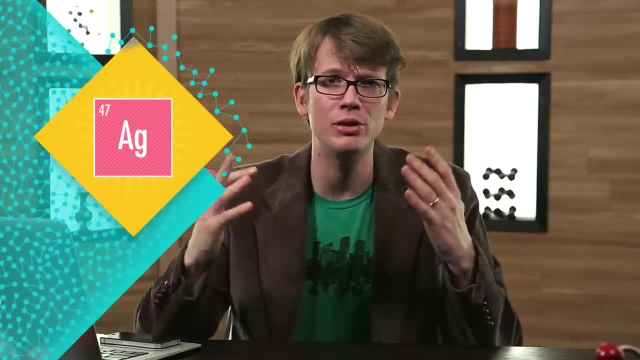 Depending on what its electrons are doing and what it's bonded to. it might be part of a chemical that's silver-colored or black-colored- Okay, this is pretty important- Or blue, or shiny, or poisonous, or a cure for disease. 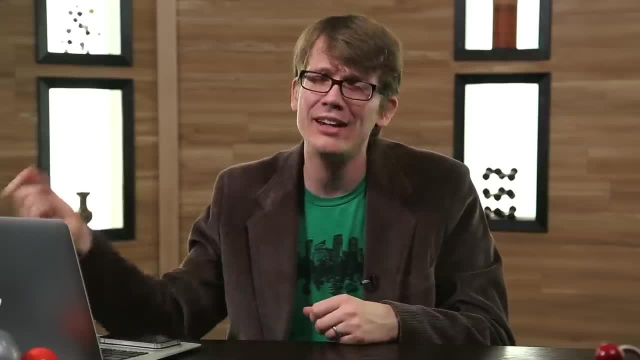 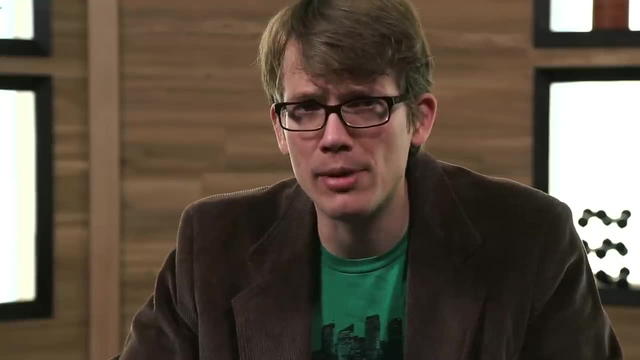 But whatever it is, that atom is still silver and will remain an atom of silver, probably forever, because that core number is very, very difficult to change. Now you might have noticed something weird about silver here. Its chemical symbol. the one or two letter short code that tells you what it is is A-G. 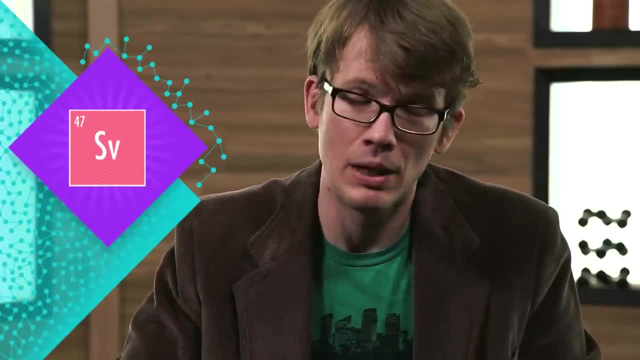 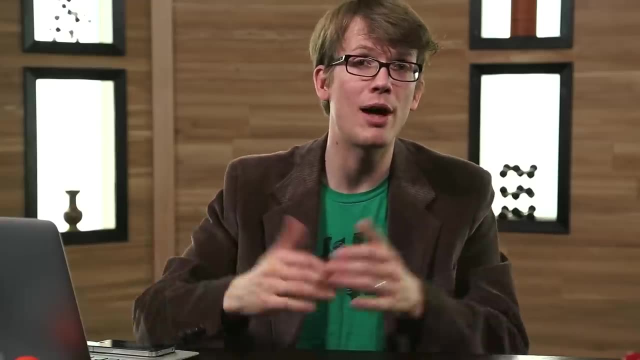 not S-I, which is silicon, or S-V, which is perfectly available, But A-G. why? To torture you? No, Silver, of course, because we've known about it for a long time, was one of the first elements. 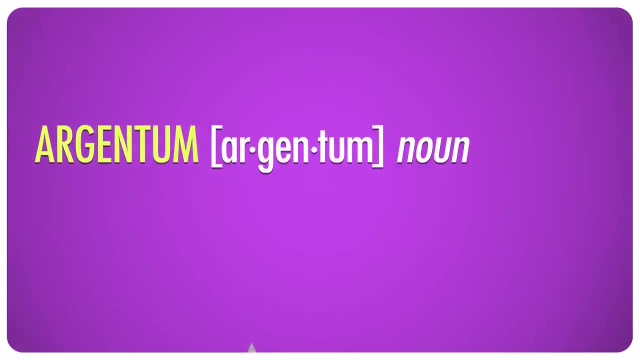 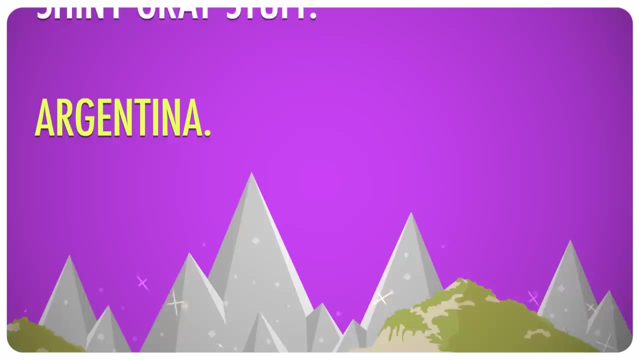 added to the periodic table and back then it was called Argentum, Latin for shiny gray stuff. Also the root of the word, Argentina, where Spanish explorers heard rumors of mountains made of silver, which of course did not exist. 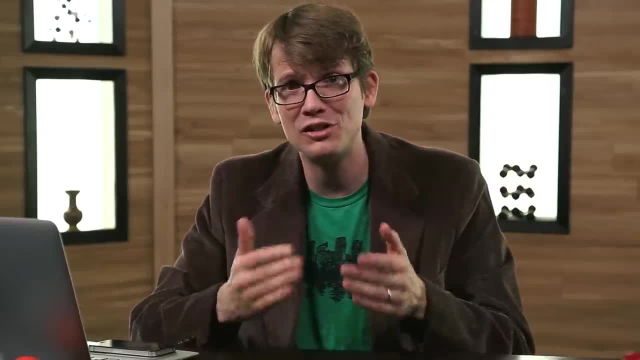 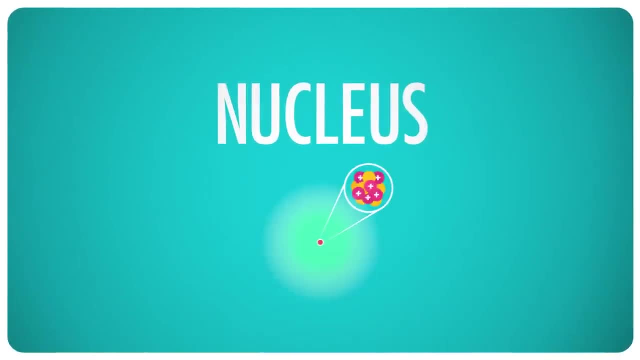 The name Argentina, just like the chemical symbol A-G stuck, despite neither of them being particularly representative of reality. Now back to science. Nuclei, which is the plural of nucleus, are boring. They're thousands of times smaller than the atom as a whole and they mostly just sit. 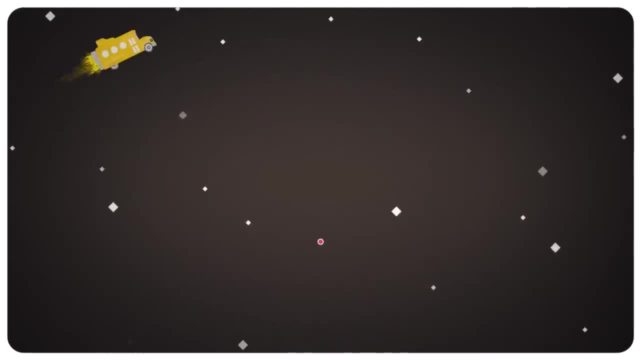 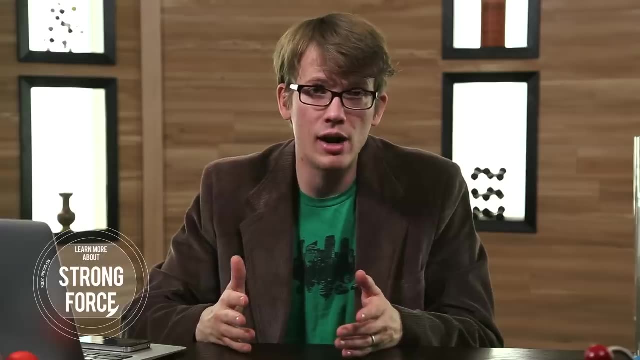 around, being exactly the same as they were when they were first created billions of years ago, held together by the strongest of the four fundamental forces of physics, the strong nuclear force. The fact that nuclei are so boring is the very reason: they're the defining characteristic. 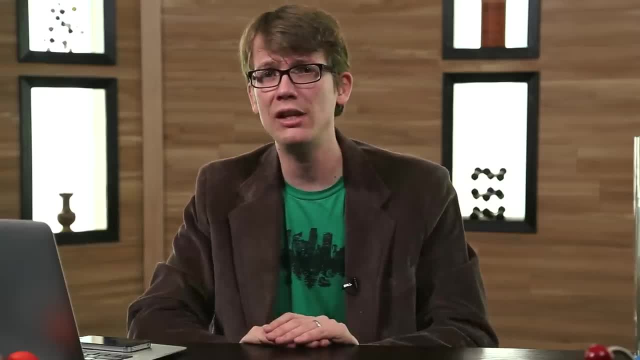 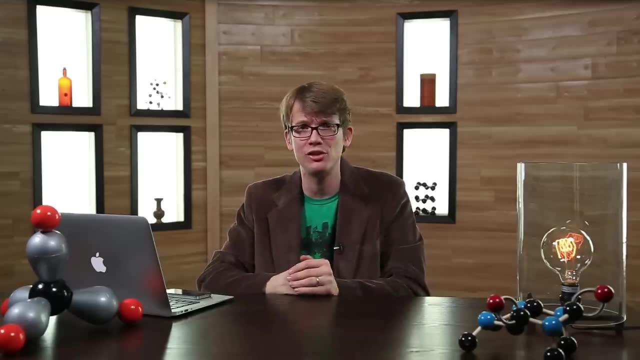 of elements. While electrons can jump from atom to atom whenever it's convenient, the number of protons is almost always extremely stable, So that core of the atom, the nucleus, always comes out of chemical reactions unscathed, The bit that we can bump around from reaction to reaction but always remains pure and 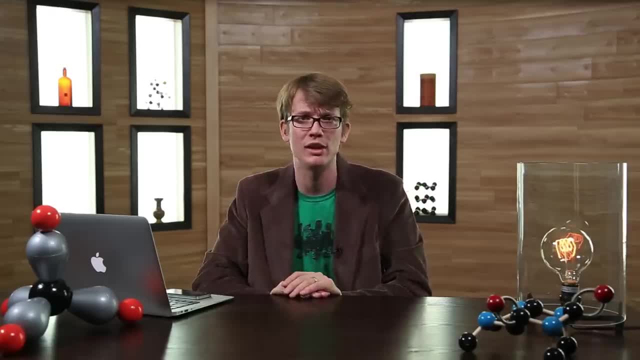 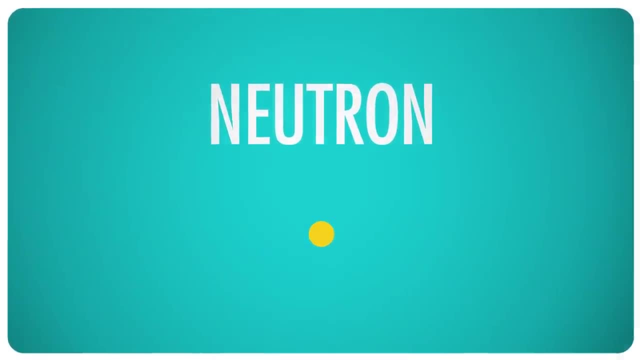 behaves the same way as any other atom with that number of protons. The atomic number is the soul of the atom. It's what makes it it. Neutrons are important too, of course, in their own way, But they don't change what element an atom is. 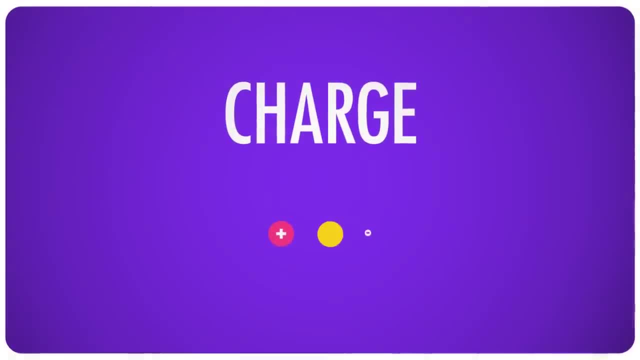 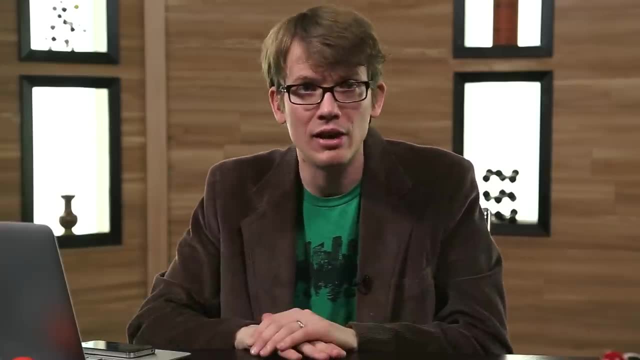 One of the two keys to all things chemical is charge. We'll discuss that in another episode. And since neutrons don't have any charge, they mostly don't change the properties of an atom, But they are nonetheless vital. We all know that, like charges repel each other. 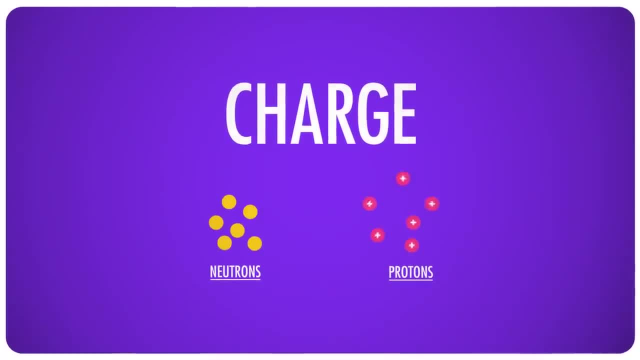 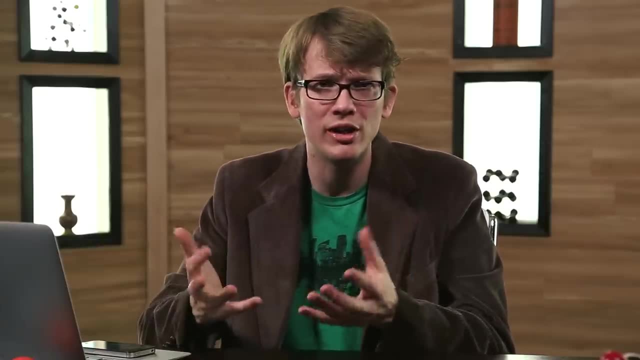 That's right. Neutrons serve as a kind of buffer between the protons. You couldn't pack silver's 47 protons together in a nucleus by themselves. They couldn't handle it, They'd rip themselves apart. So nuclei only clump together permanently when the right number of protons and neutrons 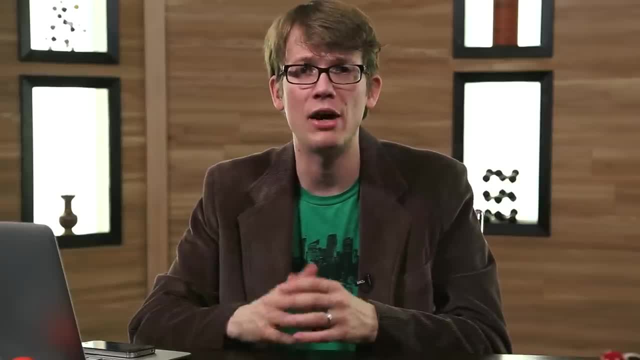 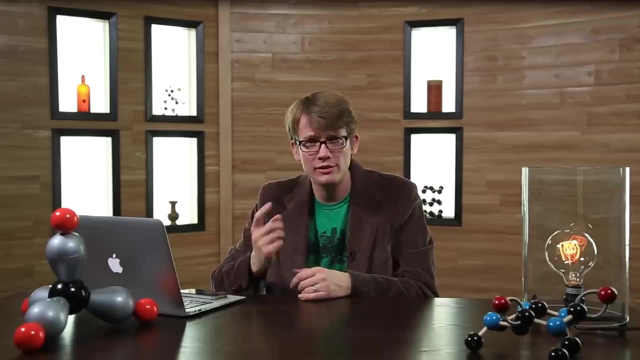 get together. Silver needs about 60 neutrons to space out the 47 protons correctly, But it doesn't have to be 60. In fact, silver nuclei are also very stable with 62 neutrons, 61, though that doesn't work. And the reasons for that I don't know, But I'll have to talk to a nuclear physicist. The atomic number of silver doesn't change as the number of neutrons changes, because the number of protons stays the same, But the relative atomic mass does change. 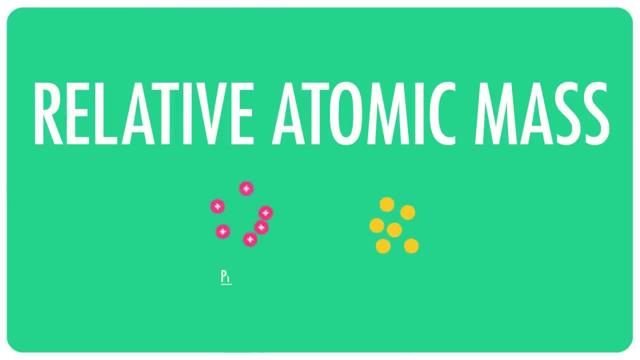 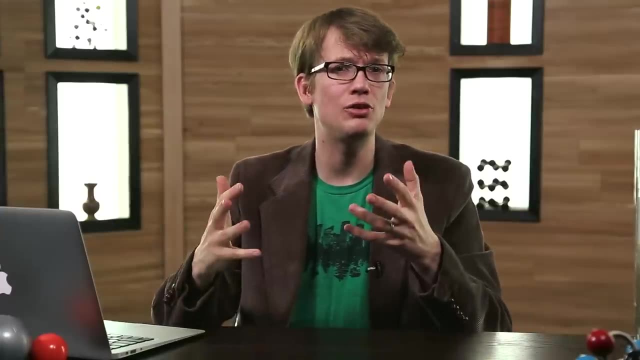 Relative atomic mass, which used to be called atomic weight back when I was in school, is basically the number of protons plus the number of neutrons averaged across all the silver on Earth, Because silver has two different stable isotopes, each with a different number of neutrons. 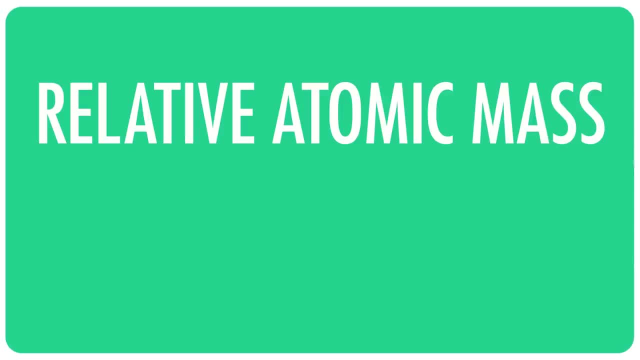 its relative atomic mass ends up not being a whole number. About 52% of silver has 60 neutrons, 88% has 62.. The relative atomic mass then ends up being about halfway between 107 and 109, 107.8682. 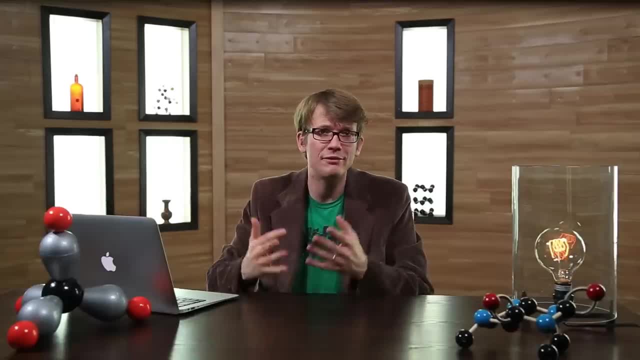 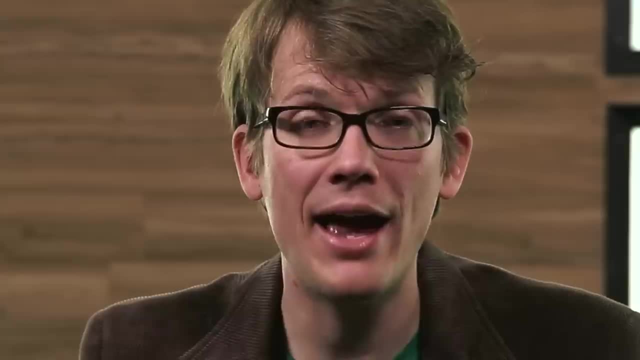 You'll note that I said these two different sorts of silver are called isotopes. They have different masses but the same chemical properties and are the same element and so belong in the same place on the periodic table. In fact, the word isotope means same place.